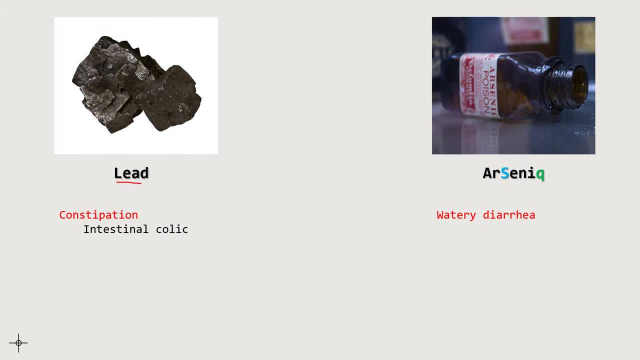 So if you know that, only that information and you can catch from the question: If you see constipation you can go on lead, And if you see water diarrhea you can go arsenic. I'm just trying to give you a practical information And 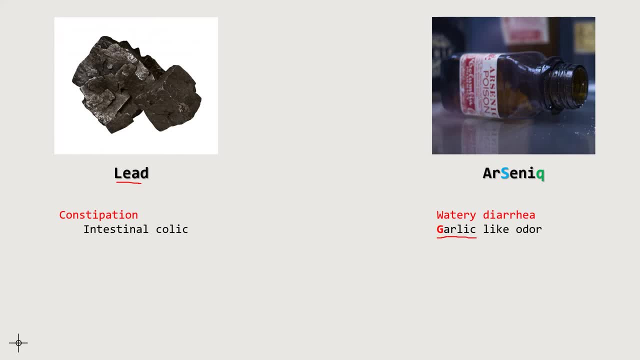 Arsenic causing garlic like odor, And this is why I always call arsenic Garsanic. Please learn that in that way, Garsanic Garsanic, causing garlic like odor, And also, As you can see, there's an S. 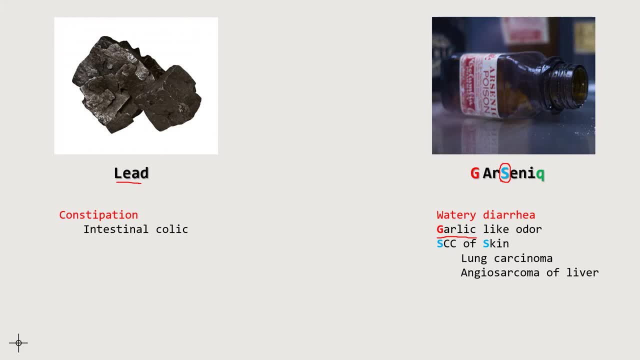 But there's no S in lead. This is Why: Because arsenic cause- I mean garsanic cause Sucomastole carcinoma of skin And also it cause lung carcinoma and angiosarcoma, Which is High yield in step one purposes. 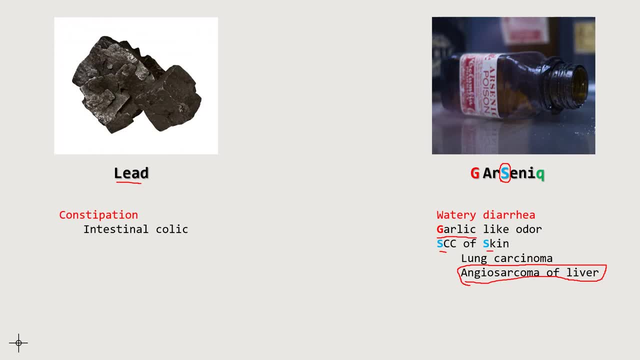 But please know, Garsanic cause a CC of skin And Also Garsanic causing cutie prolongation. So you may remember this like The last letter, Garsanic, Cutie prolongation And the last thing in comparing these. 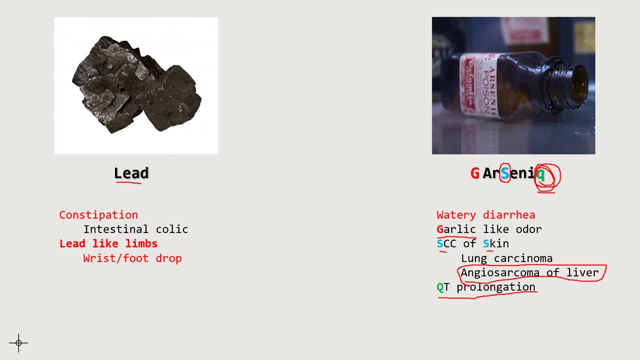 Is Lead causing lead like limbs? Lead like limbs, And what I mean for It, cause wrist and foot drop And you may even see in questions, So just saying The patient experiencing wrist or foot drops And you can go to the 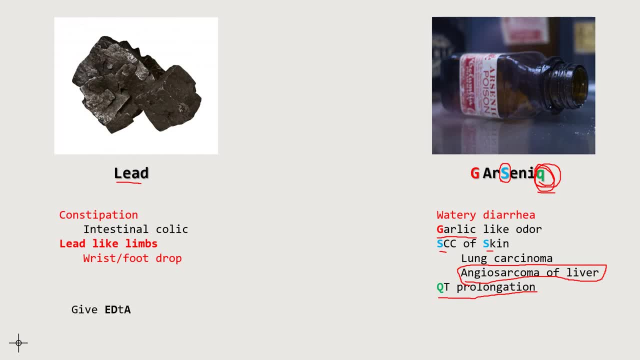 Answer as lead. Another practical thing in here is: What can we give for these patients? So we can give etta to lead poisoning? And as you can see, there is Three letters from Lead word. This is how I remember always. 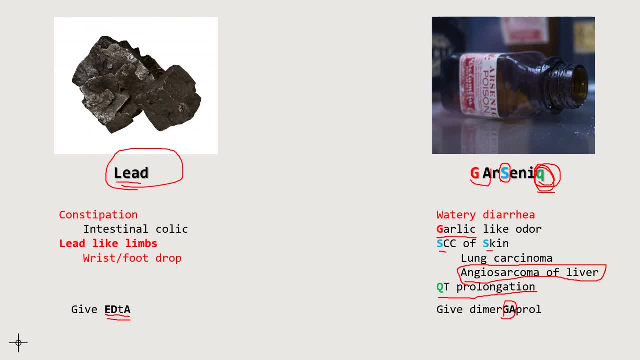 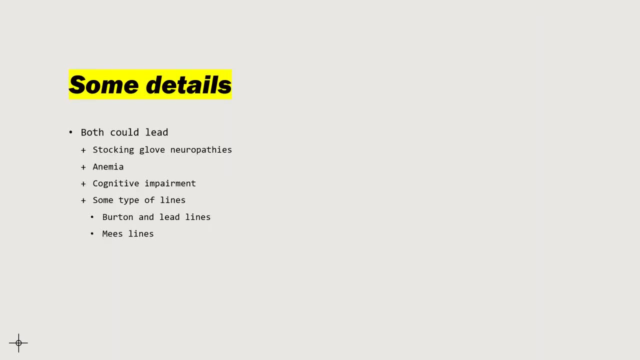 And we can give dimergaprol to Garsanic. You may see some questions in step one And There are some details that I want to talk. What could lead Stalking? low neuropathies? What could lead anemia?